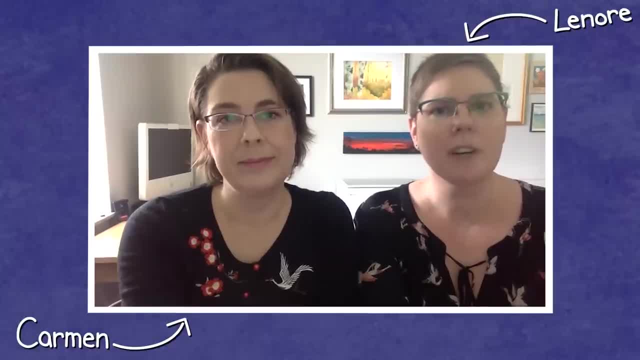 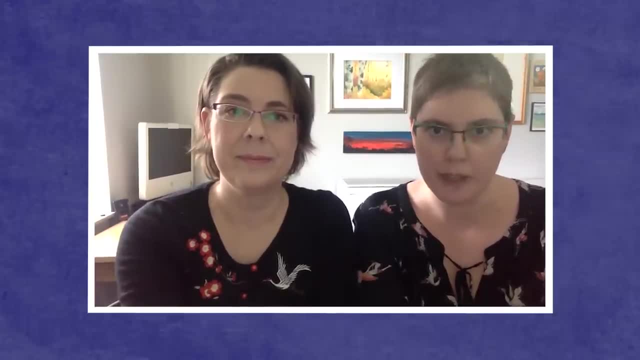 Actually, I'll let the designers explain. Just like we have different favorite colors, one person's clutter can be another person's creative inspiration. So our first step isn't to condemn clutter and get rid of it, but to figure out what you need or want in any given place. There are two main categories that we 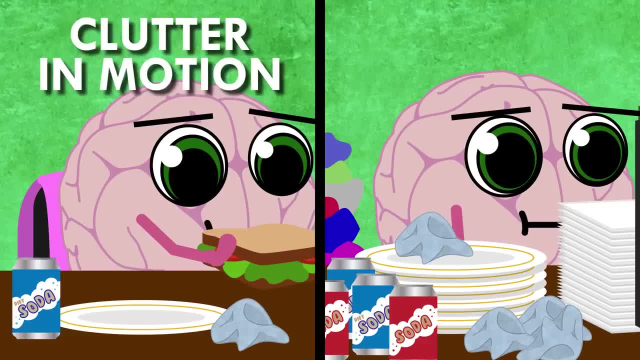 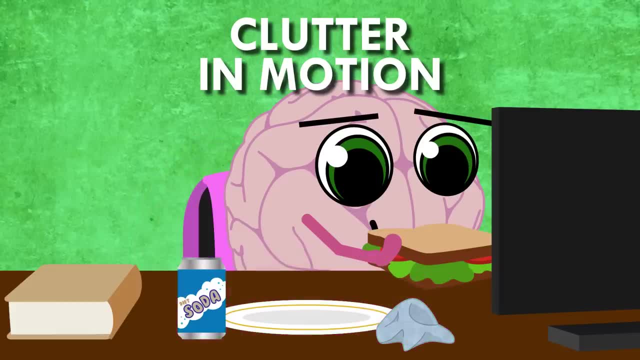 could talk about today that exist for everyone. That is clutter in motion and clutter in stasis. Living your life takes things out of place, But what we've noticed is that this sort of clutter is often tolerable or even cozy. It might look messy on an Instagram post, but it can feel good to see the 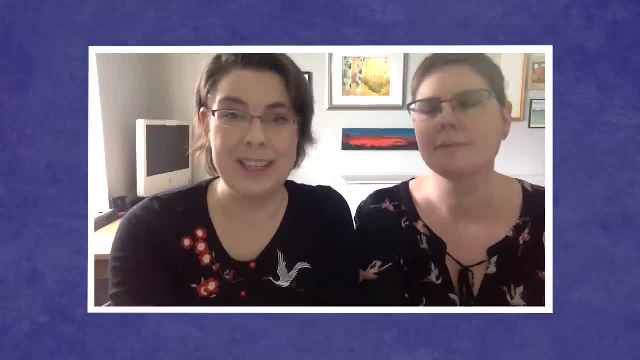 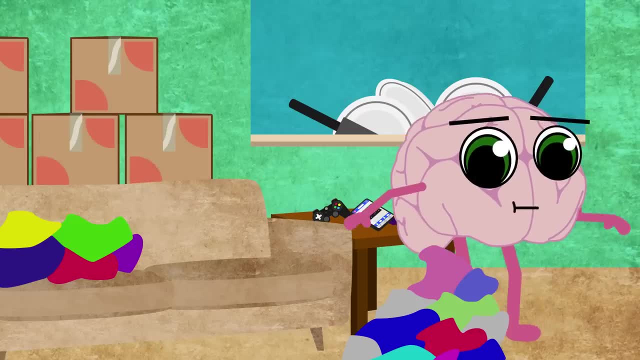 books you're reading stuck next to the couch, But there's a point where, if you don't put them away, they aren't in motion anymore. This has become clutter in stasis. So, basically, clutter in stasis is clutter that is out of place for. so 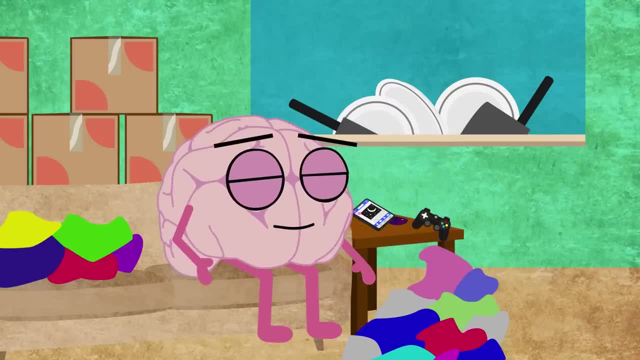 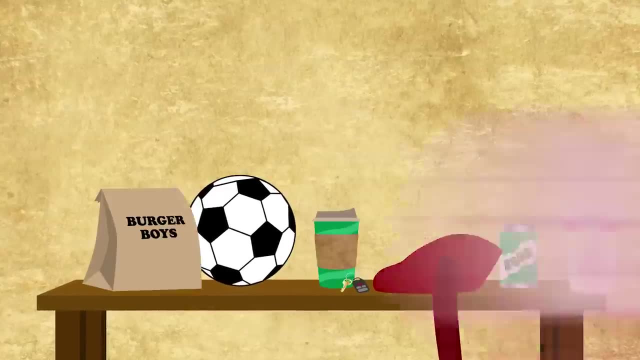 long that you've started to treat it like it's not there. You're working around it, potentially shuffling it off to the side when it's in the way It's- being treated like a permanent fixture. Sometimes clutter in stasis happens because the thing doesn't have a place. 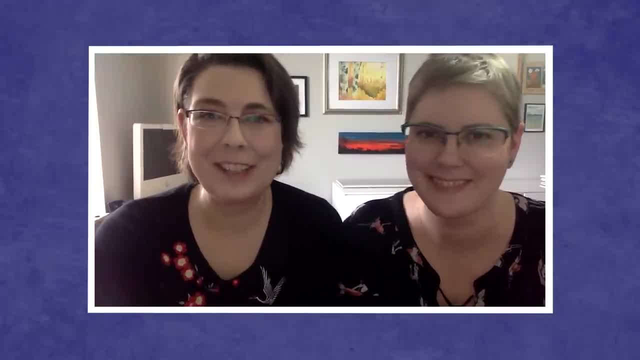 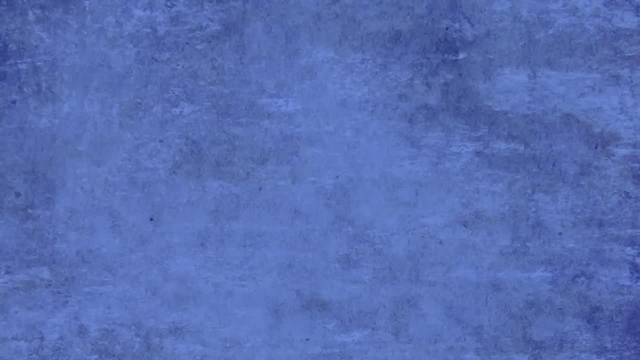 As parents. one of the major sources of this kind of clutter is the stuff our kids bring home from school: So much paper, So much art, Exactly So this can be one source of the infamous piles that so many of us have shuffling around from one corner of a closet to another. Another type of 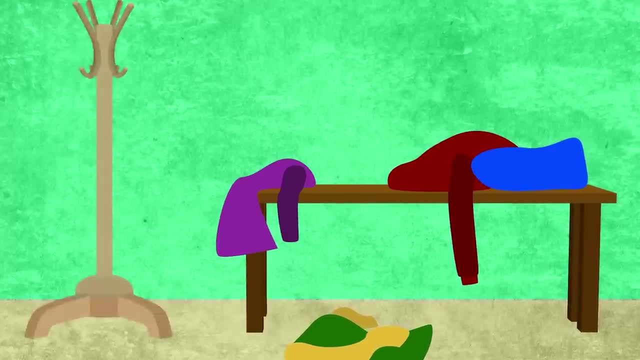 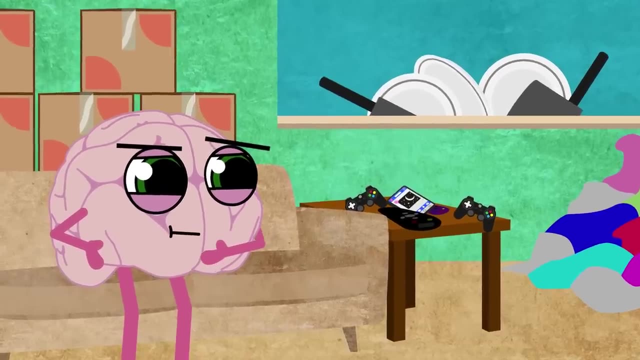 clutter in stasis comes from having a need that isn't met in that space. There's a lot you can put into place to do with both types of clutter, but the strategies are different. If you have clutter in stasis, you can ask: does this have a place and is there a? 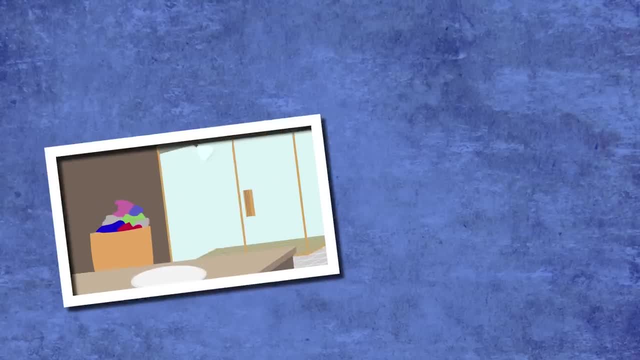 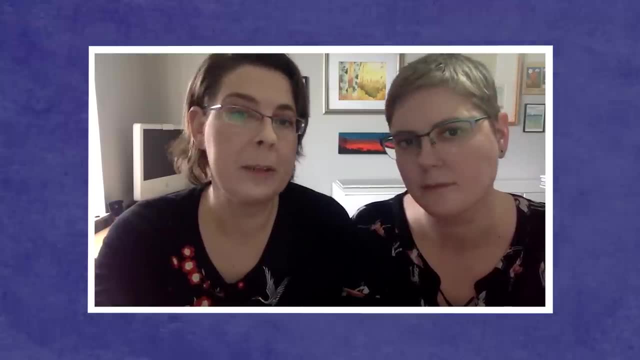 reason I don't put it there. Something as simple as a well-placed laundry basket or trash bin or a tray table that makes it easy to clear coffee cups out of the living area can have a big impact on keeping clutter in motion from turning into clutter in stasis And analyzing your piles separately from the general. 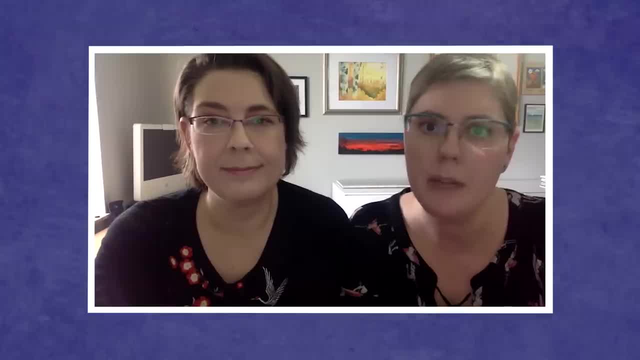 clutter can help you figure out what it is that has no place. Rather than becoming overwhelmed looking around your whole home and trying to think why everything doesn't have a place, You can simply go to your most permanent areas of mess and say what is in here. 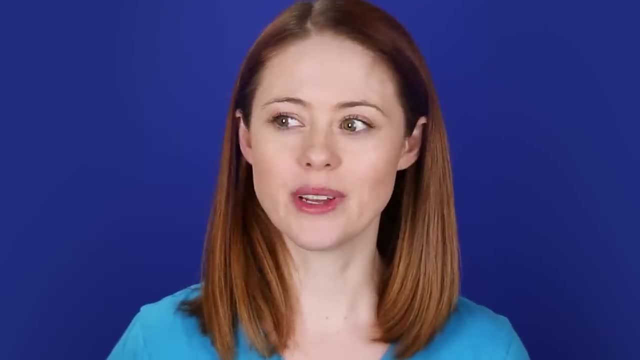 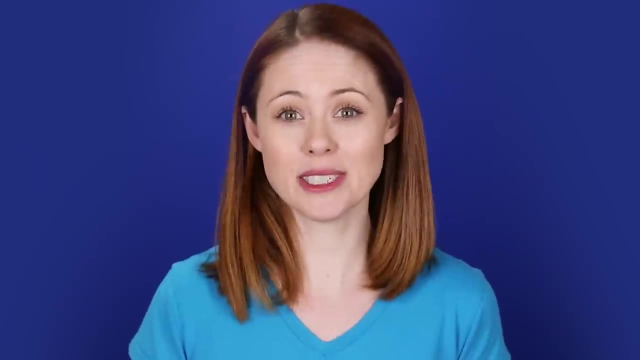 Why is it in here? It's amazing how effective this can be. So, yeah, we can't get rid of clutter completely, but we can work toward making sure that what's in our space is what we want to be in our space, And that's going to be different for.